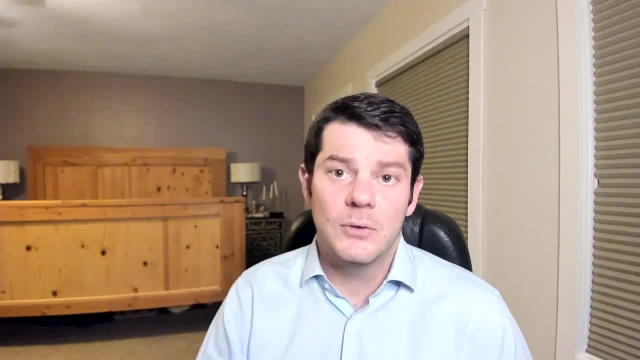 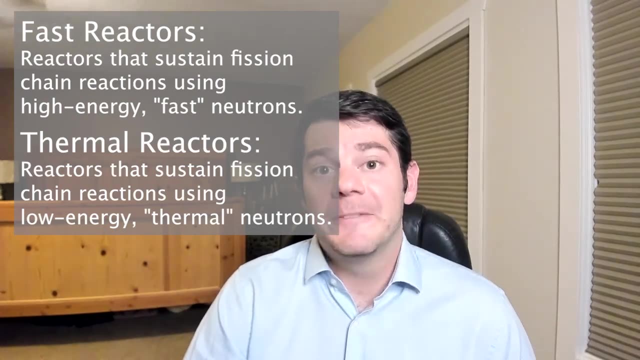 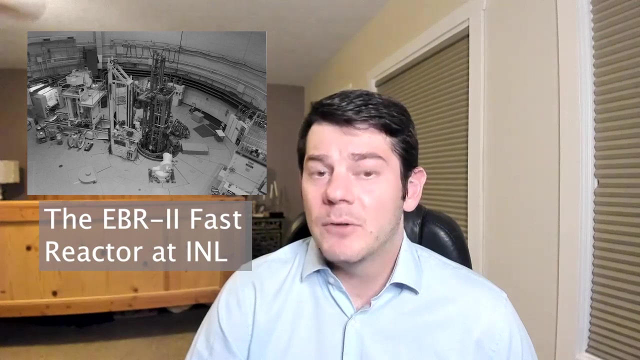 low-energy or thermal-energy neutrons to drive their fission chain reactions. So we couldn't recycle spent nuclear fuel in today's reactors but you could build fast reactors to fission all of these leftover heavy actinides. We have designed and built fast reactors before and we could gradually, and probably will- eventually transition into operating a fleet of fast reactors that run on recycled nuclear fuel. Fast reactors are also nice because you can use them to theoretically design a breeder. reactor. Nuclei will tend to release more neutrons when they fission, if the fission is induced. 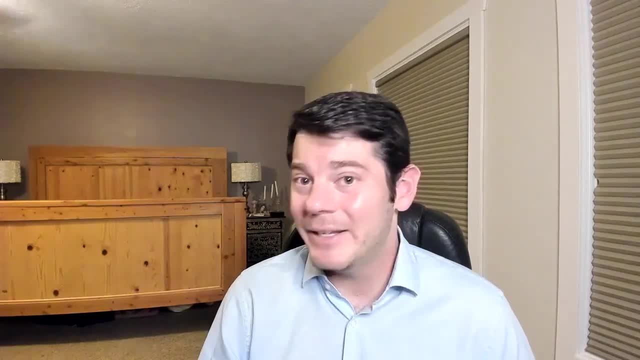 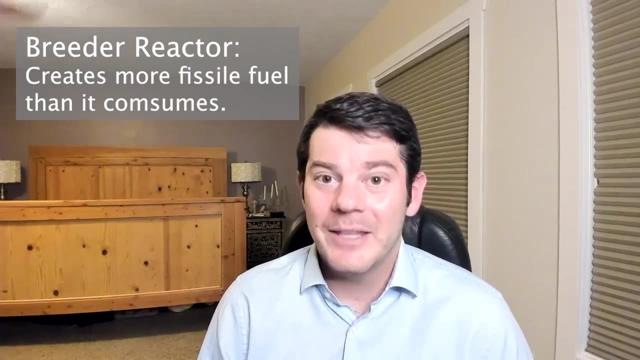 by high-energy or fast neutrons, And you can theoretically use some of these neutrons to breed fissile fuel, which means that you can create more fissile fuel than you actually consume in the reactor. As a result, you can use these neutrons to create more fissile fuel than you actually consume in the reactor. At first this sounds absurd. a reactor can't make more mass than it consumes. that violates the principle of equivalent exchange. Well, breeder reactors don't magically create mass. they instead convert isotopes that cannot fission into isotopes that can fission. 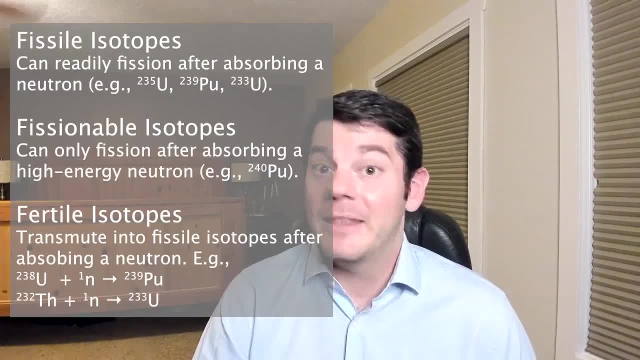 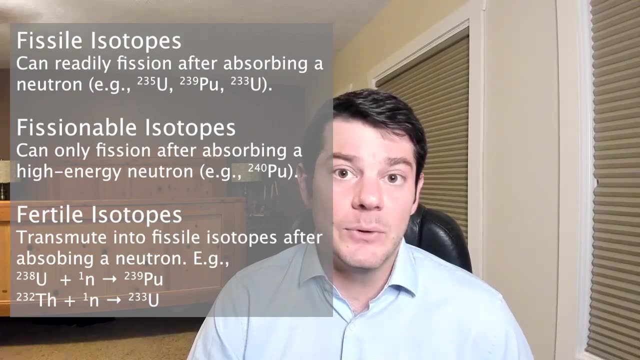 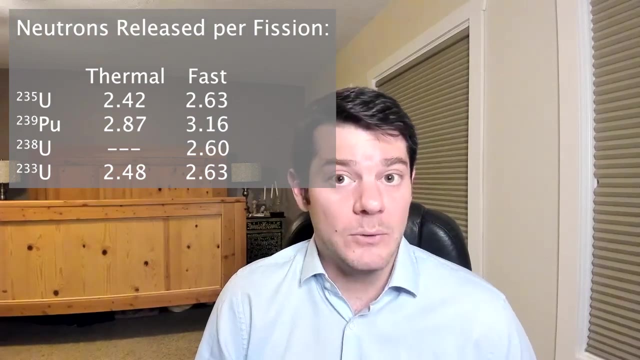 These seed isotopes are known as fertile isotopes, and they include things like uranium-238 and thorium-232,, which will transmute into plutonium-239 and uranium-233,, respectively, after absorbing a neutron, Because the average fission reaction will release more than two neutrons. you can theoretically 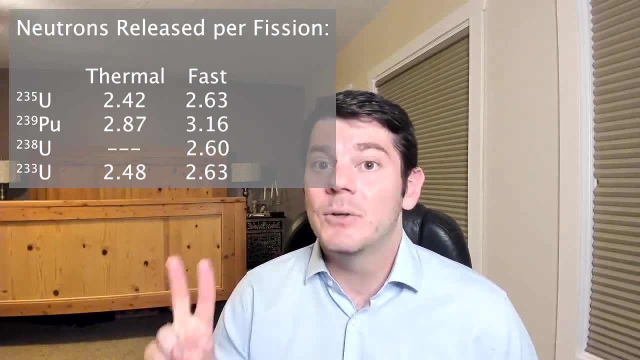 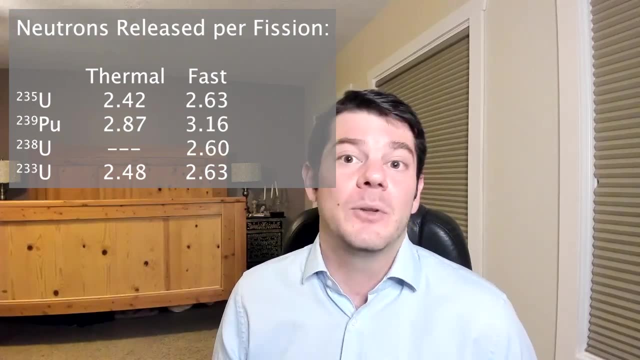 use one of these neutrons to continue the chain reaction and use the second neutron to be absorbed by a fertile isotope, thus creating a fissionable isotope to replace the one that just fissioned Breeder reactors. might sound like alchemy or black magic, but the universe conveniently. 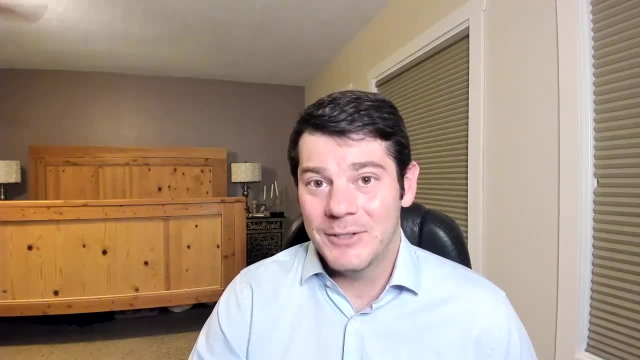 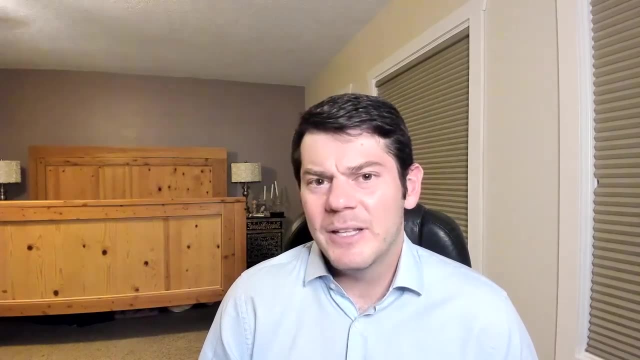 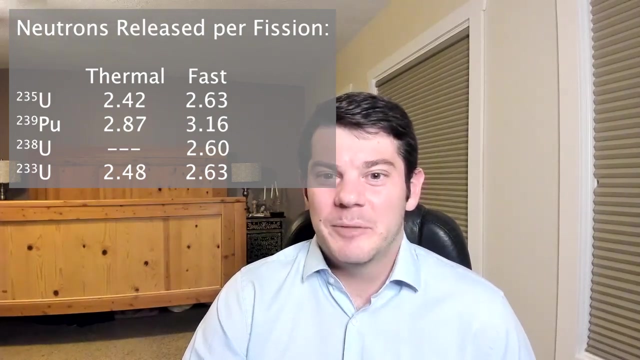 allows nuclear reactors to generate more fissile isotopes than they consume. The light-water reactors that generate more fissile isotopes than they consume are the ones that are fissionable. The uranium-235 that fuels reactors just barely doesn't release enough neutrons per fission. 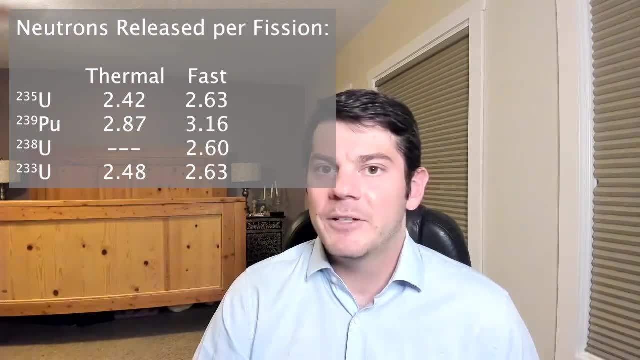 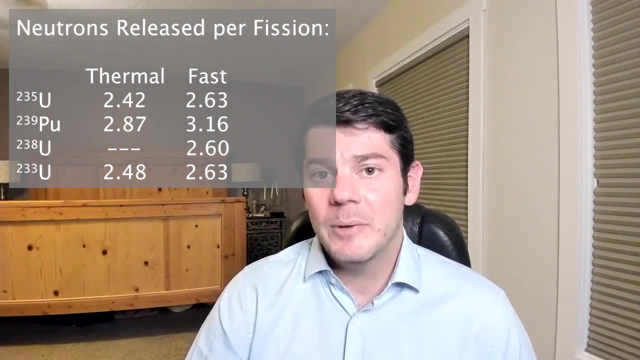 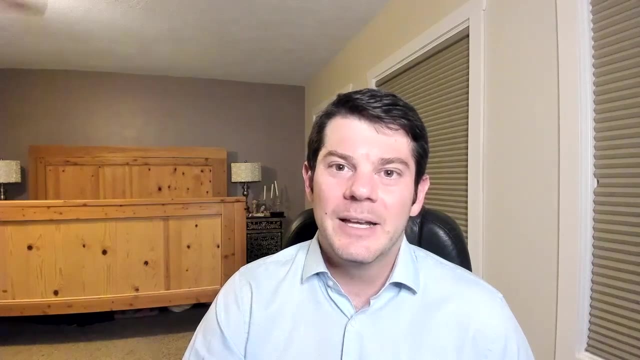 to allow for a breeder reactor design using U-235.. This means that any potential breeder reactors will likely use fast-energy neutrons with plutonium-239, or thermal-energy neutrons with plutonium-239.. The really nice thing about breeder reactors lies in just how plentiful these fertile isotopes 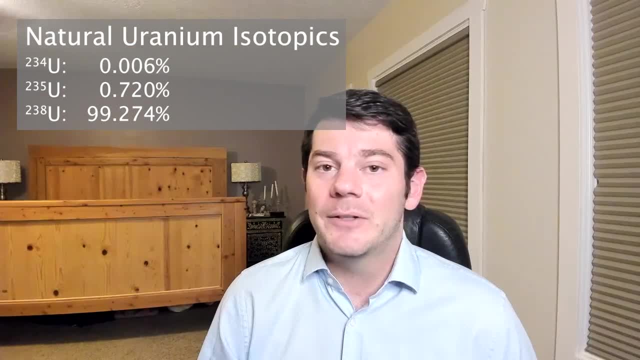 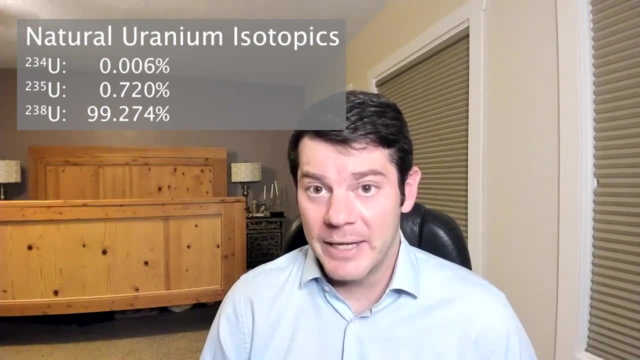 are Fissile. uranium-235 is about 0.72% of all uranium atoms, So making a nuclear reactor fuel requires mining a lot of uranium and then enriching it until it's about 3-5% uranium-235.. 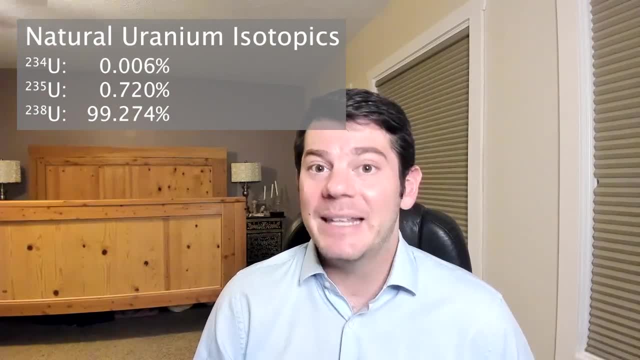 However, breeder reactors would allow us to use the remaining 99.27% of uranium-235,, which is a lot. This means that we would be able to use the remaining 99.27% of uranium-238 in our uranium by converting it into fissile plutonium-239, effectively multiplying the amount of fissile. 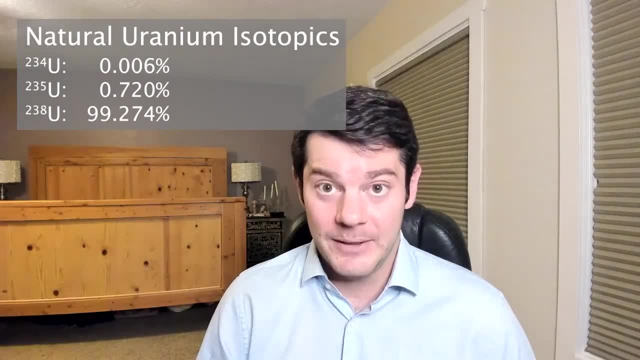 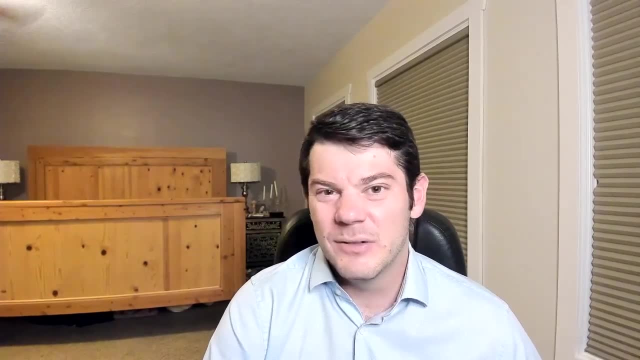 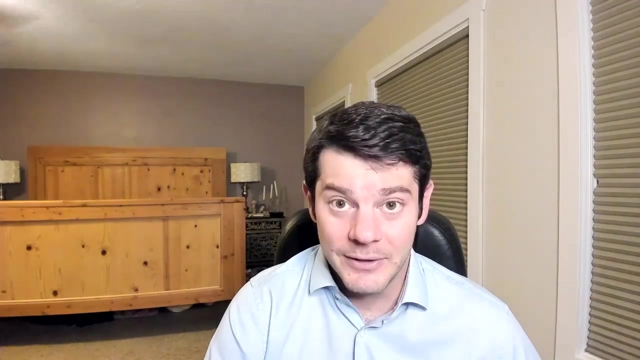 fuel that we have by a factor of nearly 150.. This is great. We have enough easily accessible uranium to satisfy humanity's energy needs for maybe the next 800 years. but with reprocessing in breeder reactors we have enough uranium to last for something like 100,000 years. 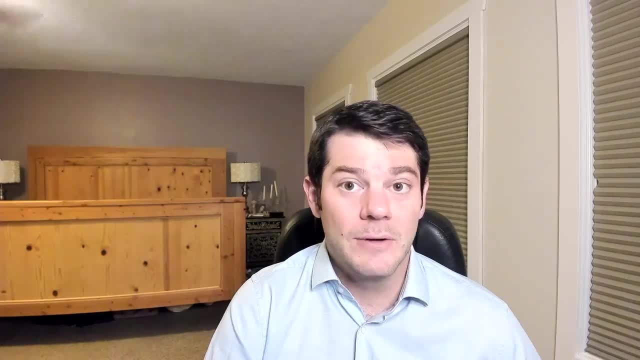 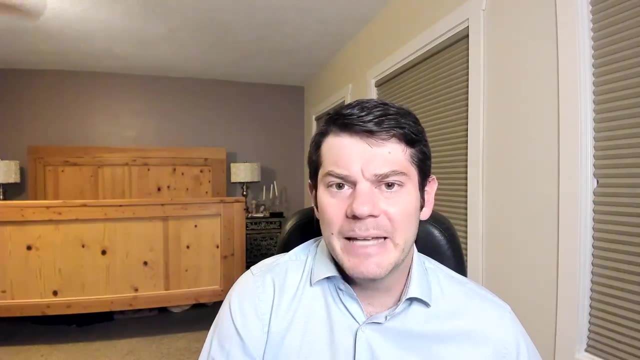 To make things even better. we don't have to limit ourselves to the amount of uranium we have. We could use thorium-232 to breed uranium-233.. Uranium is a reasonably common element. it's about as common as tungsten, silver or tin. 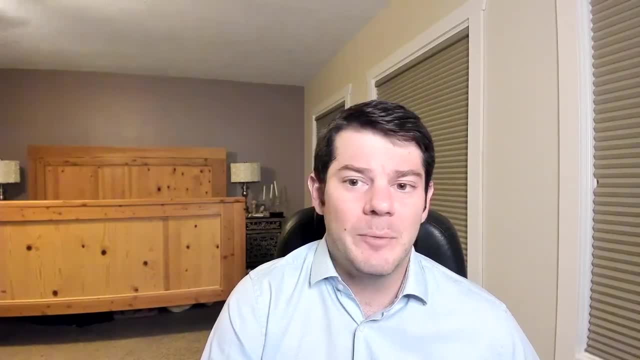 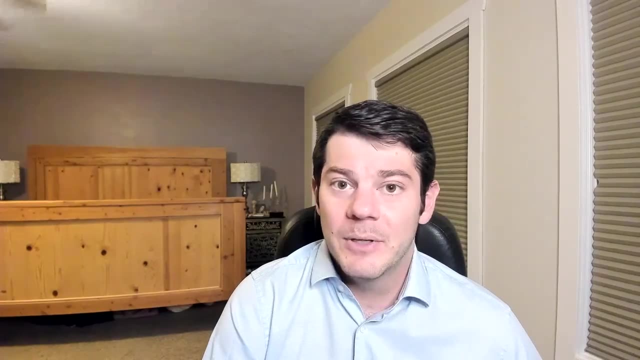 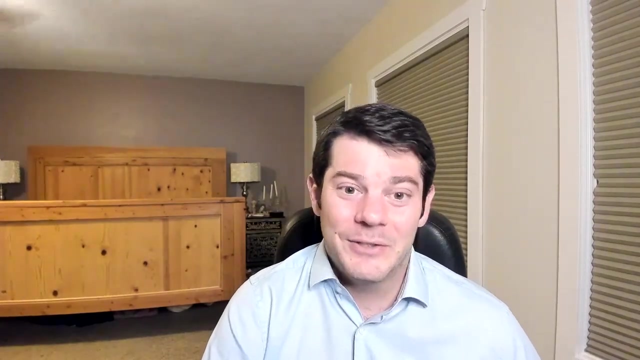 but thorium is even more plentiful. We have about as much thorium as we do boron or lead in the Earth's crust. The Earth likely has about 4 times as much thorium as uranium, which means that breeder reactors could power humanity for perhaps the next 500,000 years, which means that civilization 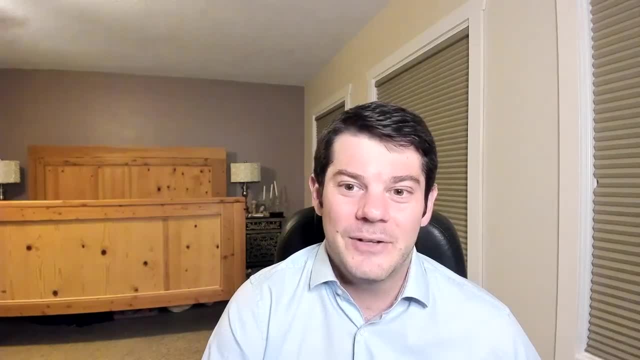 could be around long enough to see just if those crazy conservative yucca mountain dose limits hold up or not. Okay, so combining breeder reactors with chemical reprocessing allows us to recycle our fissionable isotopes and use them to produce even more energy, to the point where we can satisfy. 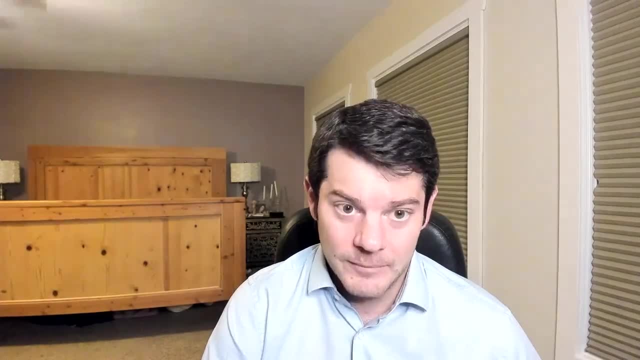 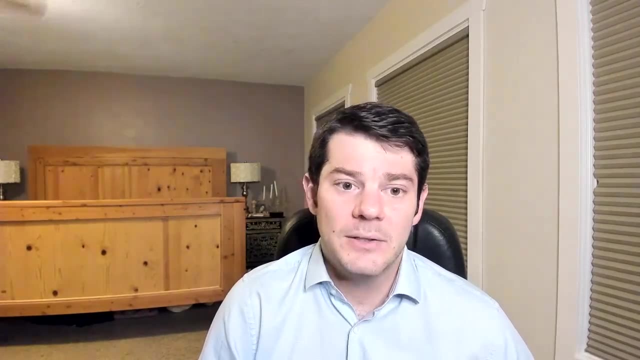 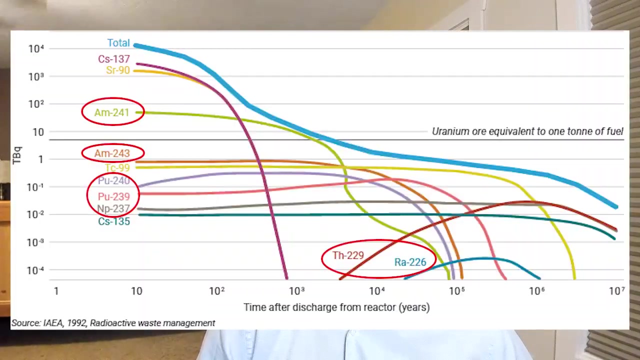 humanity's energy needs for almost the indefinite future. That's really great, but reprocessing has even more potential than that. Reprocessing also makes handling our nuclear waste much easier. So let's get started. As we discussed last time, fissionable nuclei like americium-241 and americium-243 and their 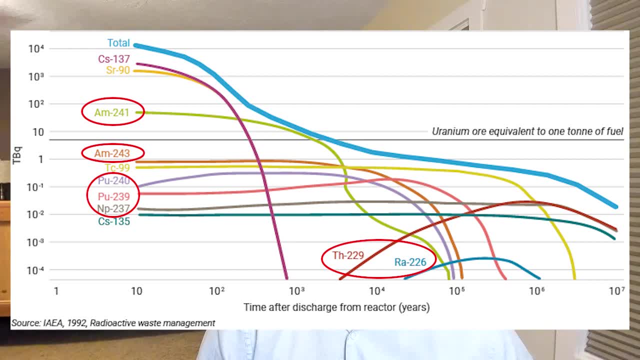 decay products are responsible for most of the long-term radioactivity in spent nuclear fuel. If you reprocess the spent fuel, you can separate out these fissionable actinides, use them to produce energy in a fast reactor, and then you don't have to worry about licensing your. 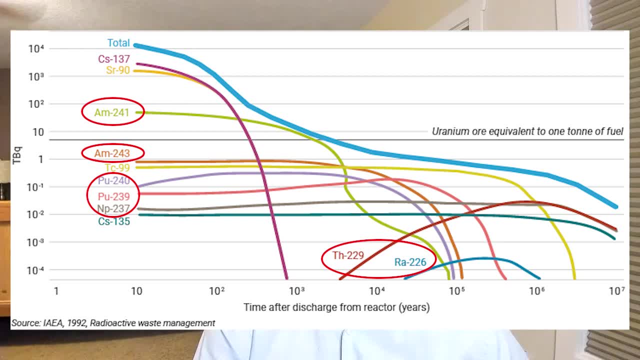 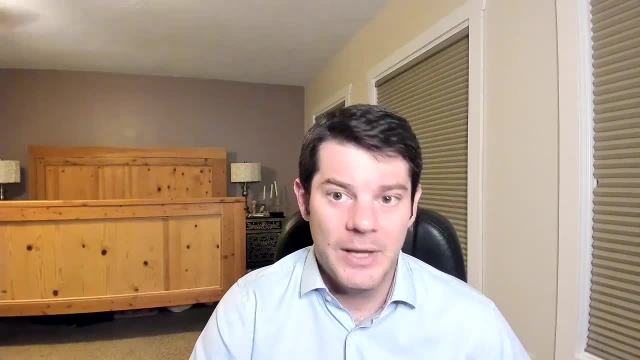 geological repository for thousands or millions of years, which is a huge deal. What's more, fissionable nuclei make up about 90% of the nuclear waste. That's a lot, And after about a decade you're left with about 95% of spent fuel. So removing these nuclei has the very minor side effect of reducing the volume of our spent fuel by 95%. So instead of having enough nuclear waste to cover one football field, you now have to dispose of enough nuclear waste to cover only 5% of one football field. 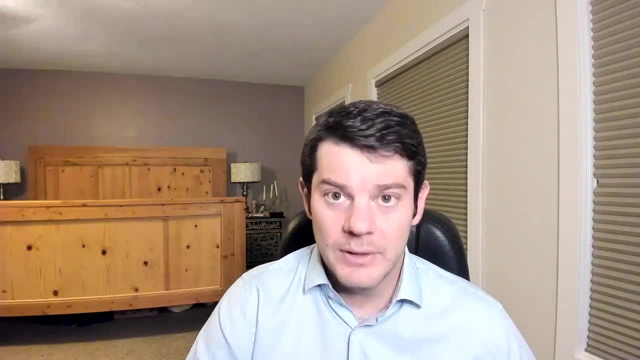 Reducing the volume of our spent fuel by 95% is a huge deal. All of a sudden, we have plenty of space in Yucca Mountain to store the remaining waste and technically we can save it, And that's a huge deal. But we don't have enough space in the Yucca Mountain to store the remaining waste, And so if it's a huge deal, we use the small amount of waste we have and we'll save the rest of the waste for the rest of the year. and techniques like deep borehole disposal, that aren't really economic for large volumes of nuclear waste, all of a sudden become way more feasible. Okay, so let's say that we reprocess our spent nuclear fuel and 95% of it is recycled in fast breeder reactors. So what do we do with? the remaining 5%. Again, this 5% is made up of fission products, which are still radioactive but are generally much easier to handle than longer-lived heavy actinides. It turns out that a lot of these fission products are incredibly useful for medical procedures: Technetium-99,. 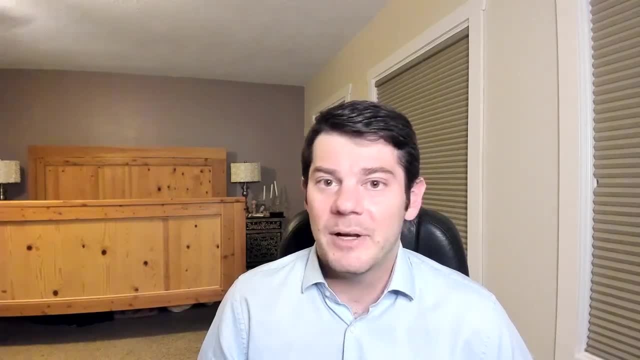 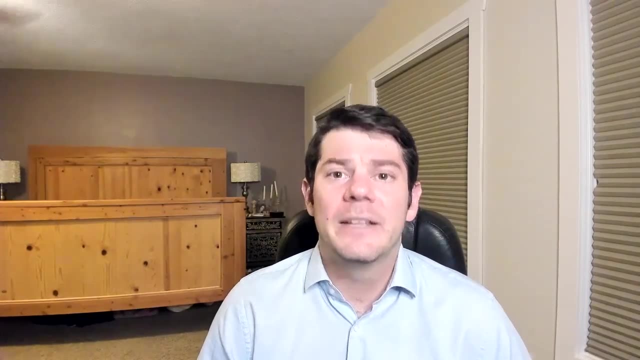 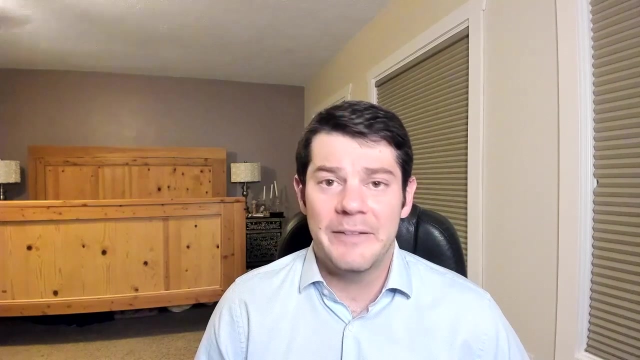 for example, is used for heart scans, and it is a decay product of molybdenum-99.. All isotopes of technetium and its precursors have a relatively short half-life on a geological scale, which means that they were not present on Earth in any significant quantity before the advent of fission. 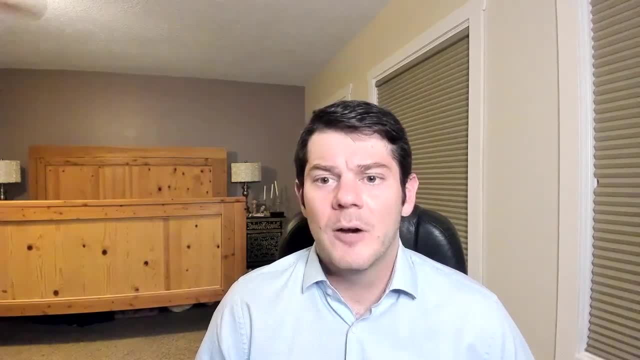 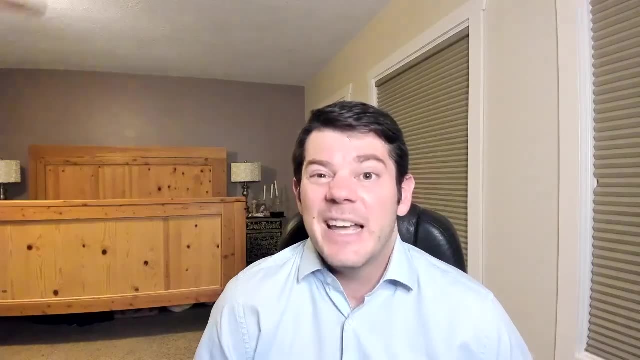 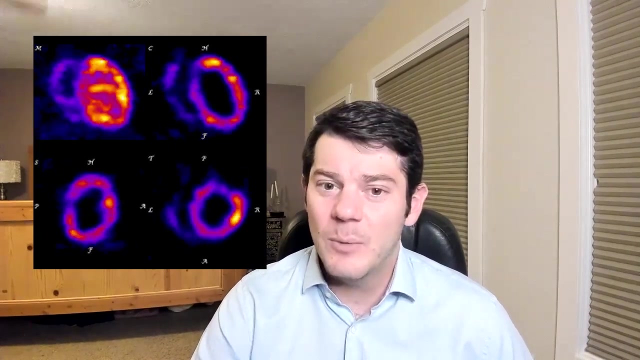 reactors Because there was no technetium on Earth. our bodies have not evolved to use technetium for any biological processes, which means that our bodies just excrete any technetium that is injected into our bloodstream slowly over time. This makes technetium-99 an excellent isotope for 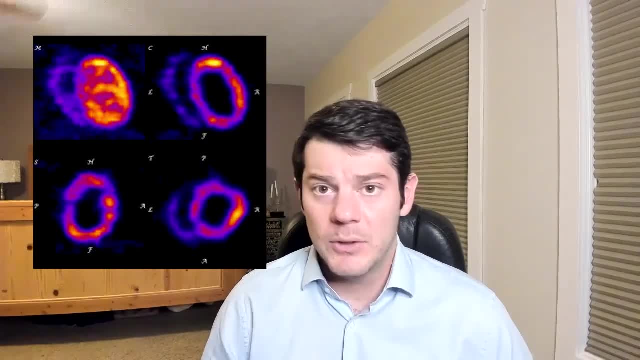 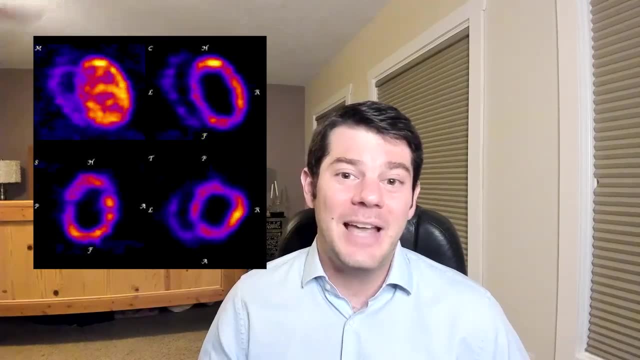 mapping, artery blockage and heart function. What you do is you inject technetium-99 into a patient's bloodstream, you sit them in front of a radiation detector and then you get to see exactly where the technetium and where their blood is or is not flowing. Because of this, technetium-99 is worth. 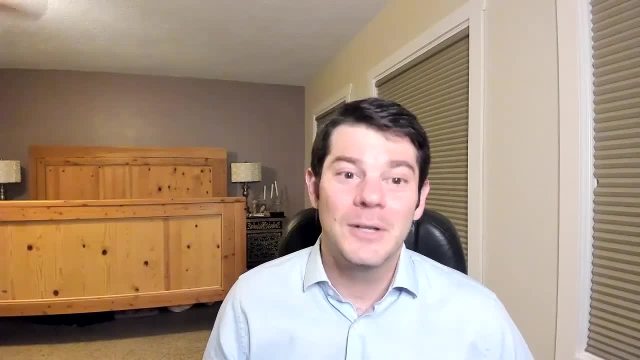 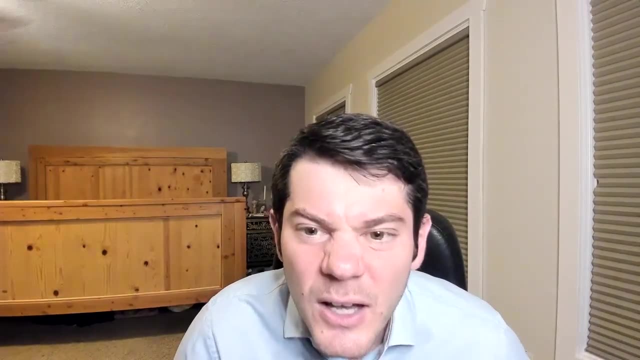 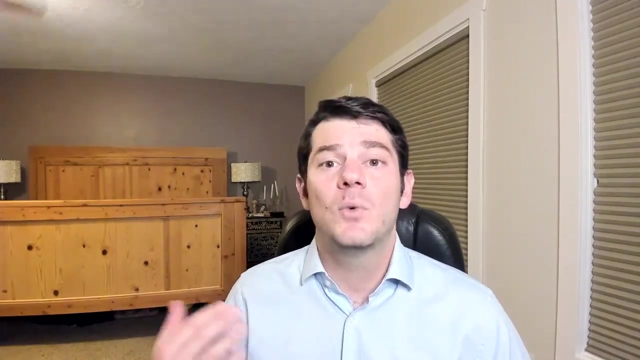 gold. Actually, that's not quite true. Gold is worth about $65 per gram, while technetium-99 is worth about $3 billion per gram. So I guess technetium-99 is worth its weight in technetium. This is just. 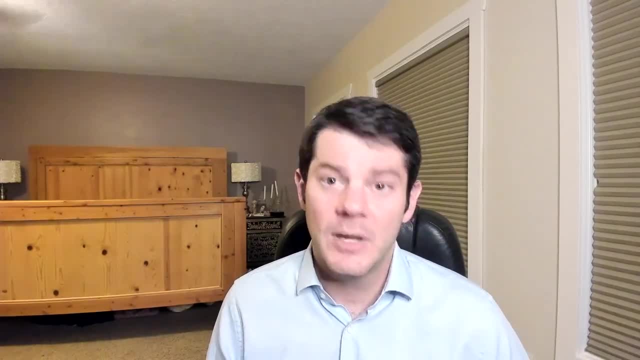 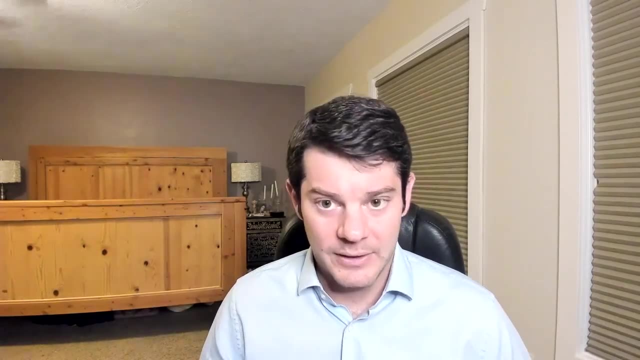 one example of medical applications for radioisotopes. There are plenty more. For example, you can also attach radionuclides to glucose, and with radiation detectors you can see what parts of our body are consuming radionuclides. This is just one example of medical applications for 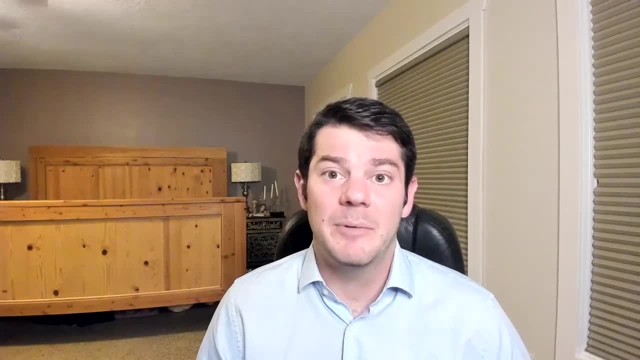 radioisotopes. The radiation detector, however, does not give you the information that the radioisotopes are consuming a host of radionuclides. This means that blood is actually accumulating a host of radionuclides, which is what you may want to be learning in a training session or training. 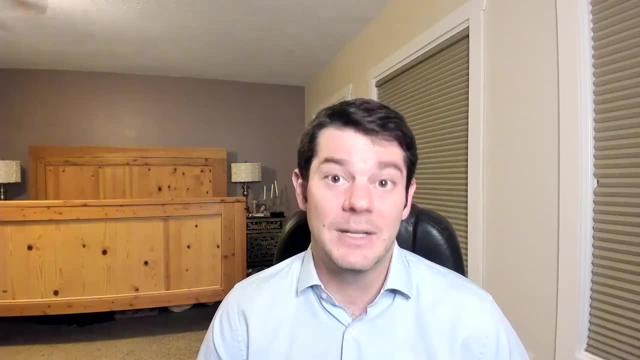 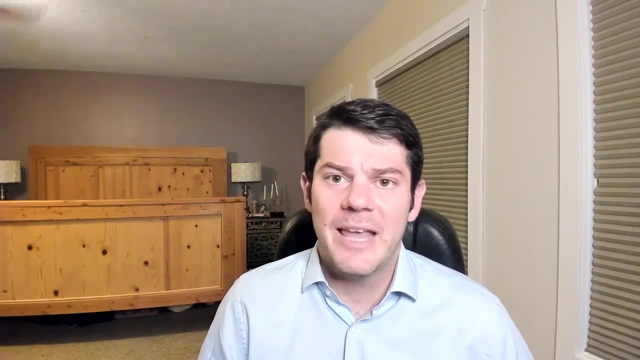 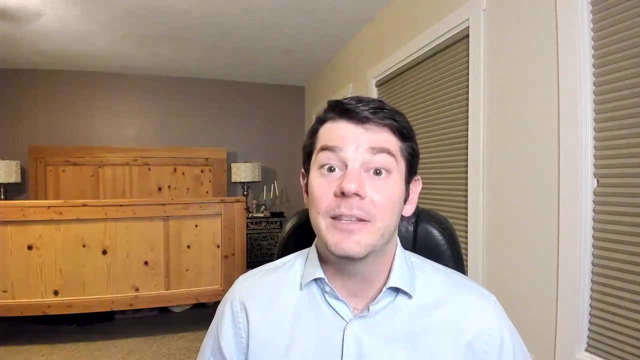 program. Cancer cells are extremely metabolically active, which means that they consume glucose like crazy, which means that you can identify cancerous tumors by attaching radioisotopes to glucose and using radiation detectors to look for these glucose consumption hotspots, them in collateral damage. This is where radioisotopes come in If you crank up. 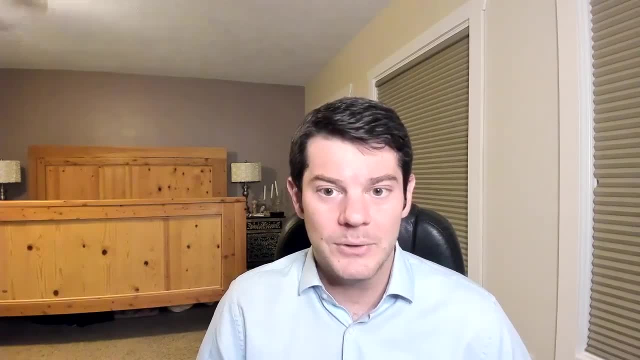 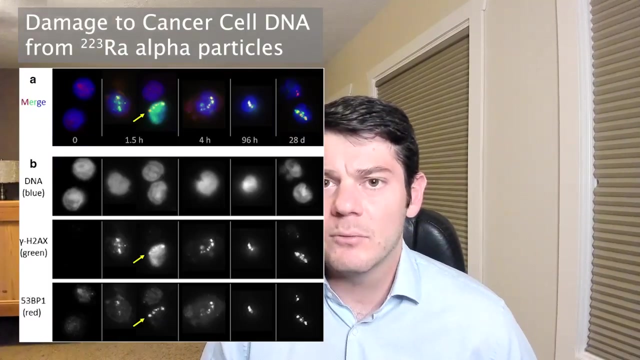 the activity of radioisotopes that are attached to the glucose molecules, then you can deliver a lethal dose of radiation to the metabolically active cancer cells while more or less sparing the surrounding healthy cells. Some types of radiation, such as alpha particle radiation, have an extremely short range. 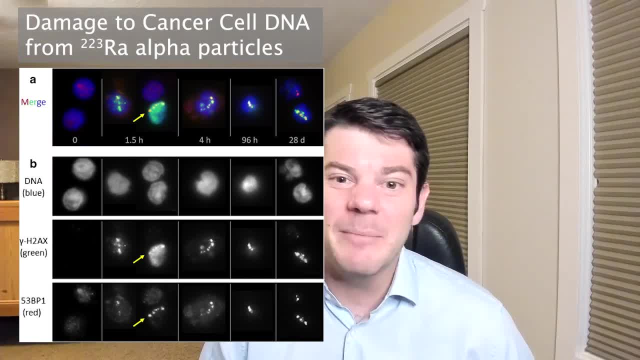 Alpha particles have a range that's on the order of about 50 microns in tissue, and the average cancer cell is about 10 to 20 microns in radius, which means that the alpha-emitting radioisotopes attached to glucose will pretty much 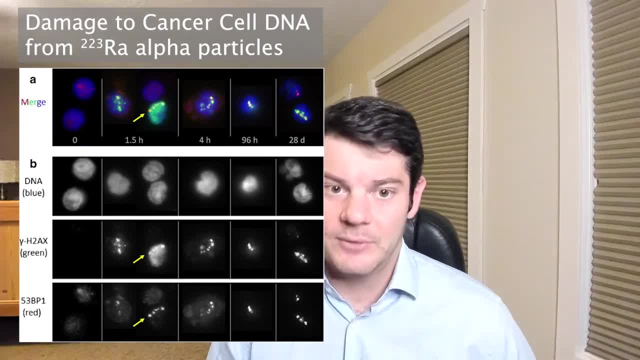 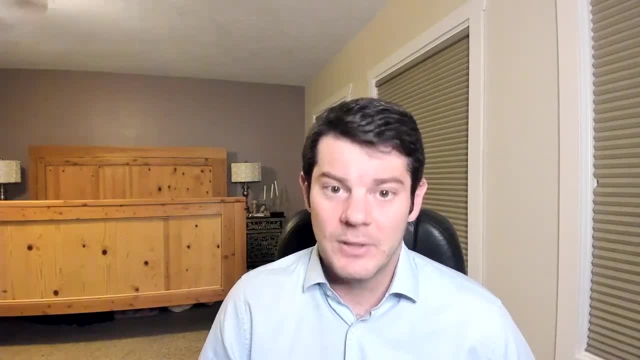 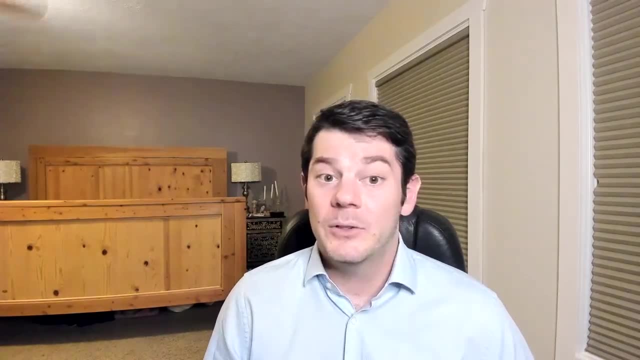 only damage the cancer cells that gobble up the glucose. There are tons of medically valuable isotopes in spent nuclear fuel and we're actually in the middle of a huge technetium-99 shortage, and reprocessing spent fuel would provide a sustainable source for these medically necessary isotopes. So after you recycle the fissionable isotopes in fast reactors. you're going to be able to recycle the fissionable isotopes in fast reactors and you're going to be able to recycle the fissionable isotopes in fast reactors. extract the medically useful isotopes from the remaining 5% of the fission. 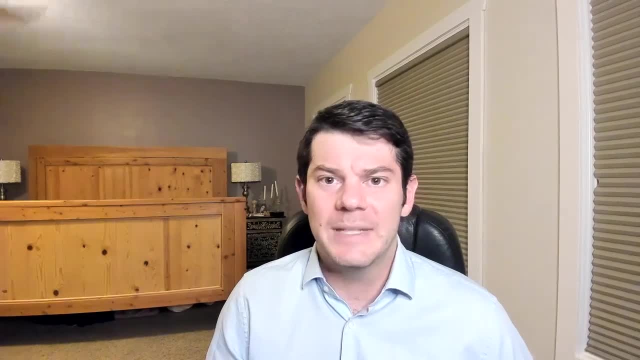 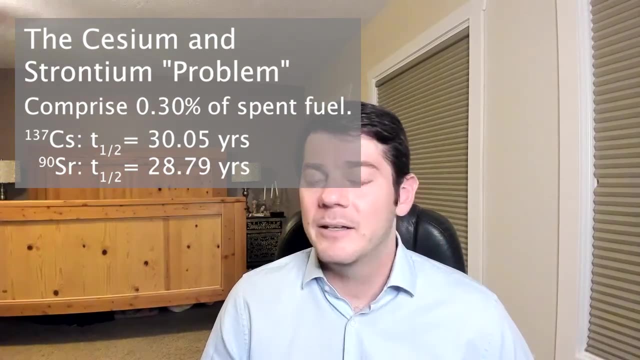 products and you wait for the various short-lived radioisotopes to decay away. then what do you have left? You pretty much only have cesium and strontium left after that. Cesium and strontium comprise about 0.3% of spent nuclear. 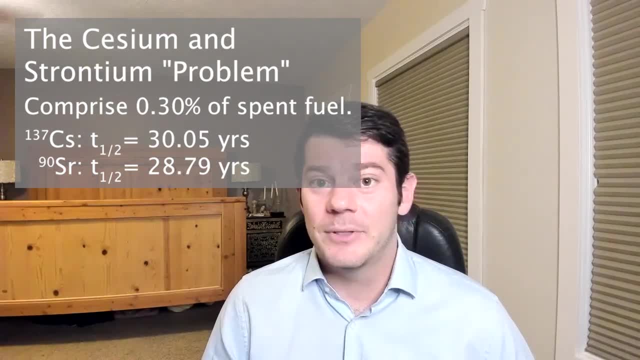 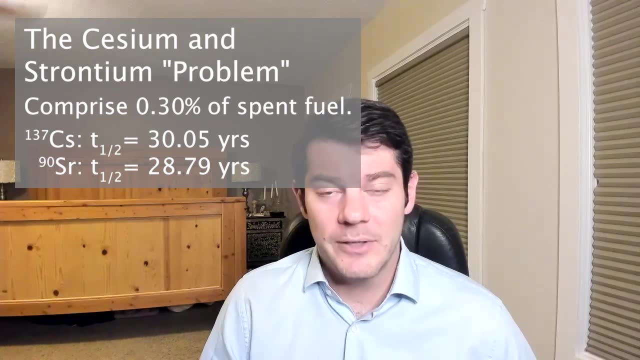 fuel, which means that reprocessing our fuel has reduced its volume by a whopping 99.7%. As I discussed in the first video in this series, we don't actually have a ton of spent nuclear fuel to dispose of but, after reprocessing fast reactors, extracting useful isotopes for medical 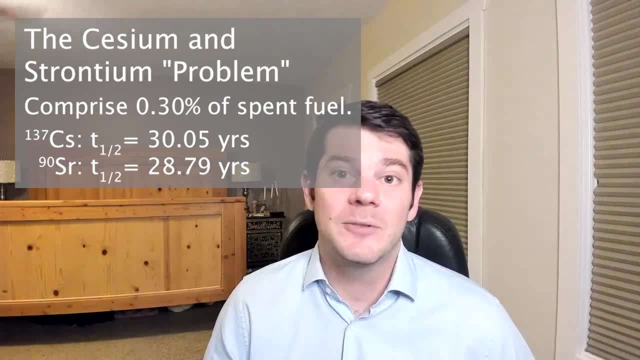 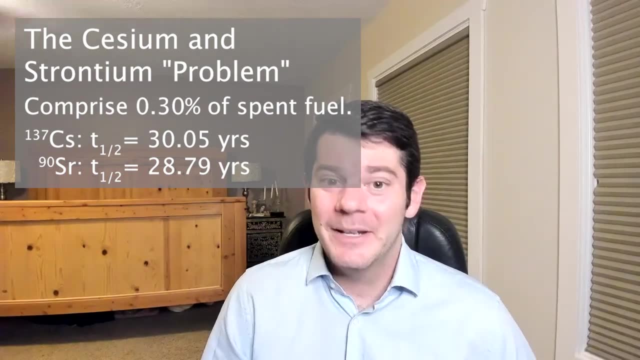 and industrial applications, then we only need to dispose of a small fraction of our original waste, about 0.3%. To make things even better, disposing of cesium and strontium really isn't that difficult. Both isotopes have about a 30. 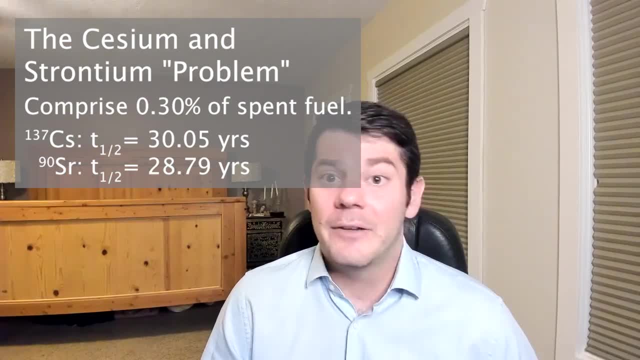 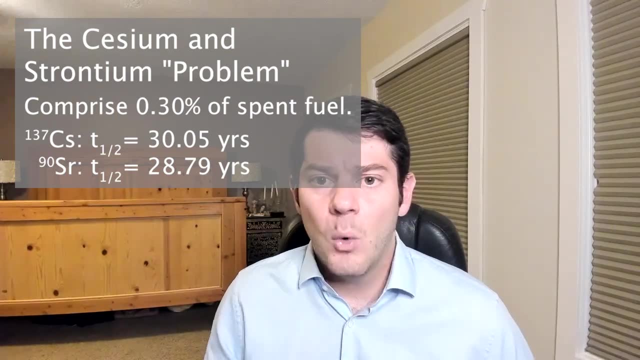 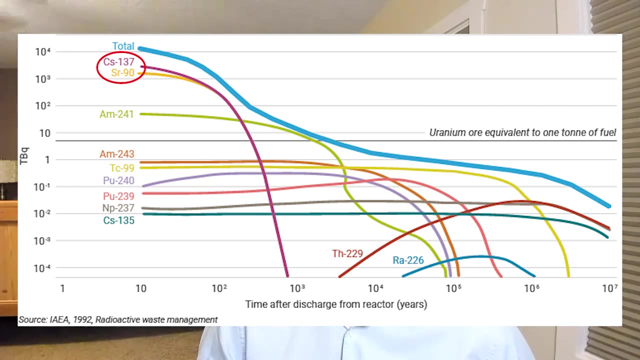 year half-life and they decay into daughter nuclei that are either stable or are very quickly stable. As a rule of thumb, radioactive nuclei are generally considered 100% decayed after about 10 half-lives, which means that disposing of cesium and strontium requires building a waste disposal site that can hold these. 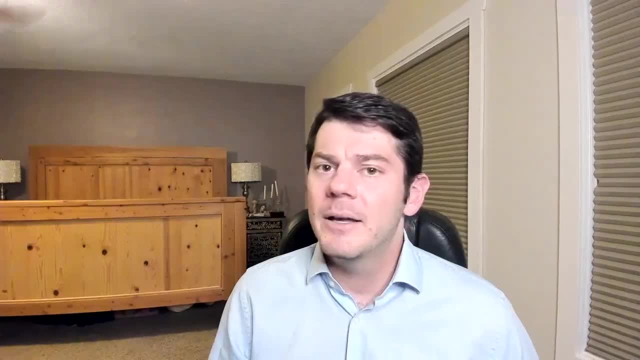 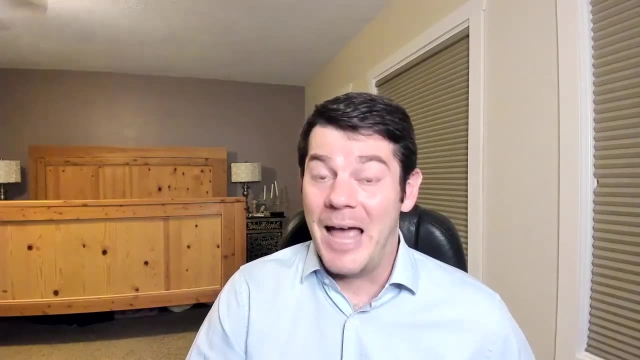 isotopes intact for about 300 years. So can we build a structure to hold cesium and strontium waste for 300 years? Yes, we absolutely can. 300 years might sound like a long time for you and me, but actually it's an extremely short amount. 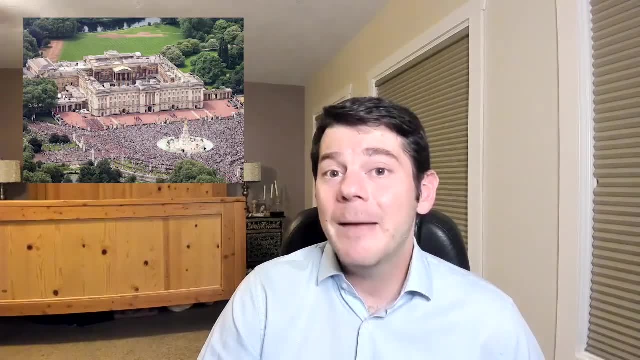 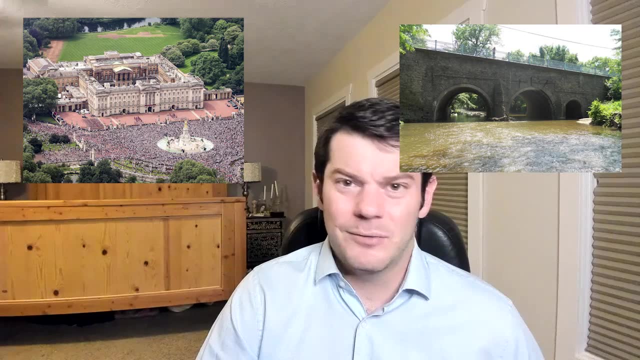 of time. on a construction engineering time scale, Buckingham Palace was built in 1703, which means that it has been around for more than 300 years. This random bridge that I found on Google is the Frankford Avenue Bridge in Northeast Philadelphia. It was built in 1697, and it's doing just fine. I mean, aside from 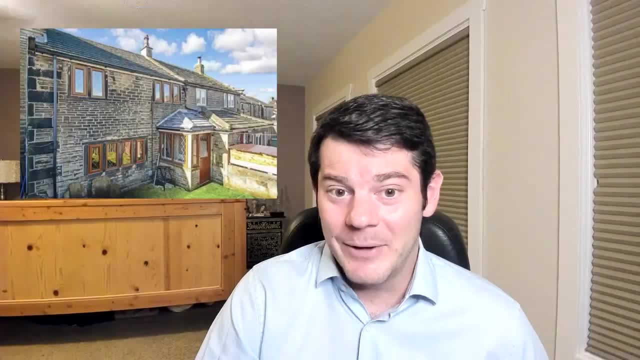 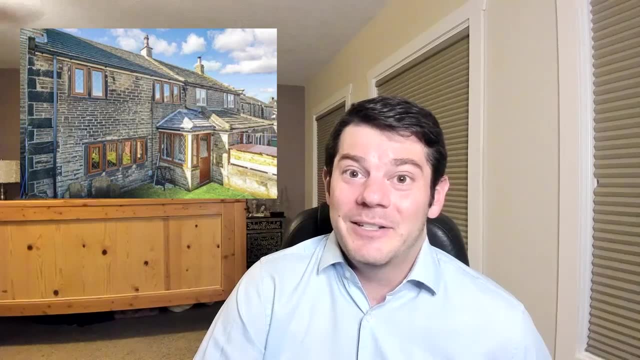 the fact that it's in Philadelphia. This 500-year-old house went up for sale in the UK a few years ago. It even has its own sauna, which is probably a great place for storing cesium and strontium. The United States is a fairly young. 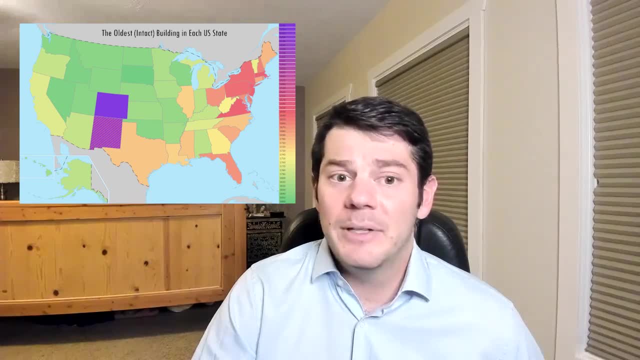 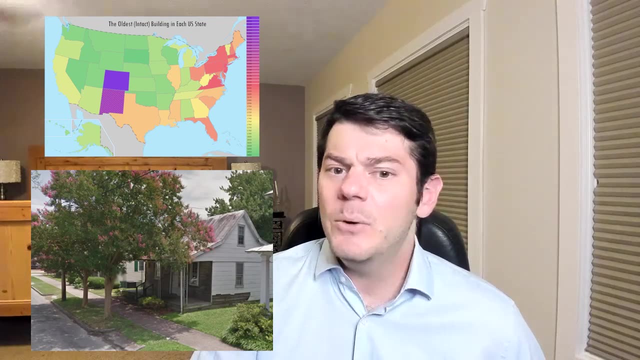 country, but a fair number of states in the US contain buildings that are more than 300 years old, including the Lane House in Edenton, North Carolina. The owners of this house, Steve and Linda Lane, were remodeling their house in 2013. 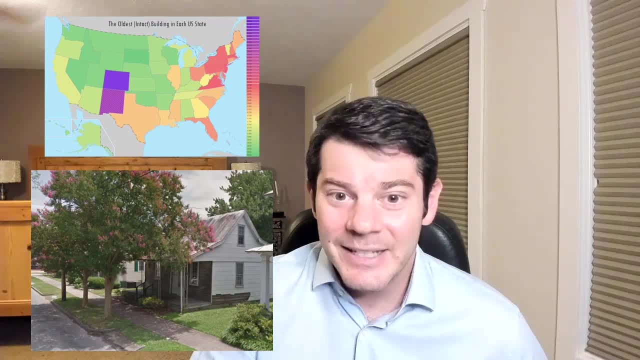 when they discovered timber from 1719 that was concealed behind cheap plastic walls- The house was built in the late 18th century and was built in the early 19th century- They had absolutely no idea that they were living in a home that was. 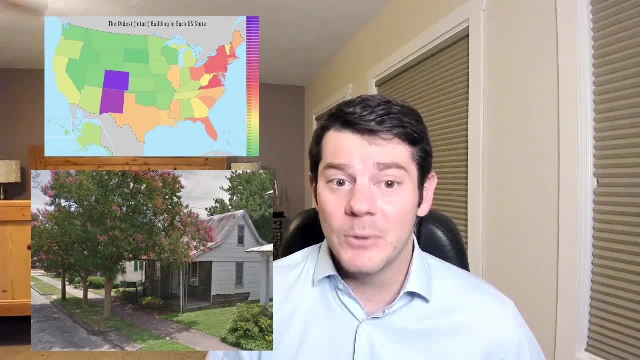 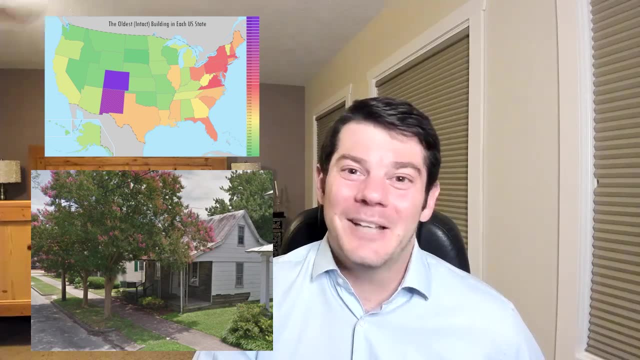 more than 300 years old, and that was actually the oldest building in North Carolina. If these folks can accidentally live in a house that's more than 300 years old, then the $44 billion that we have stashed away in the Nuclear Waste Fund can certainly engineer a structure to safely. 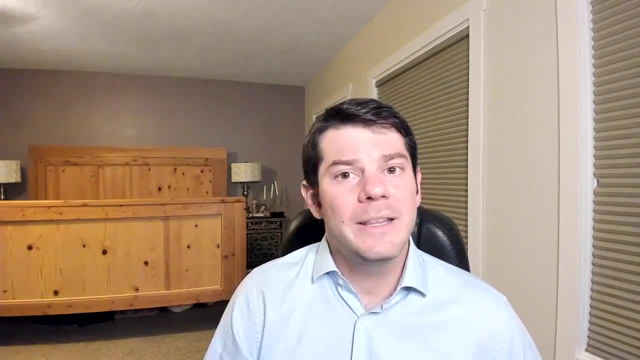 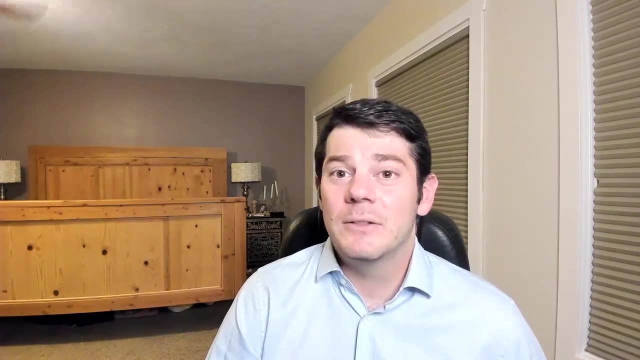 house our nuclear waste for 300 years. So what are the downsides to reprocessing our waste? First and foremost is economics. Right now, it's actually cheaper to mine new uranium, enrich it and fabricate it into new fuel than it is to recycle our old fuel. This economic reality will not always be the case. There is a lot of uranium out there, but we will eventually start running low on it and we'll need to start reprocessing and recycling our spent nuclear fuel. This won't happen for maybe about 800 years, but we will run out of. 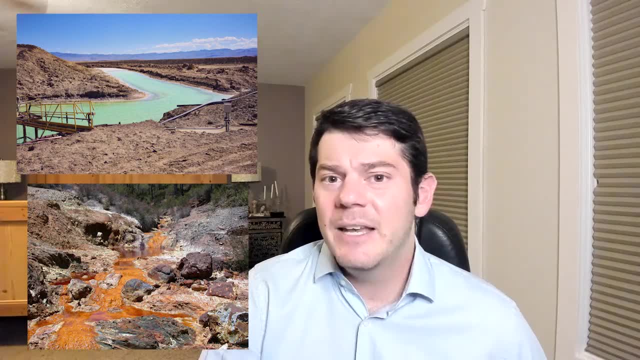 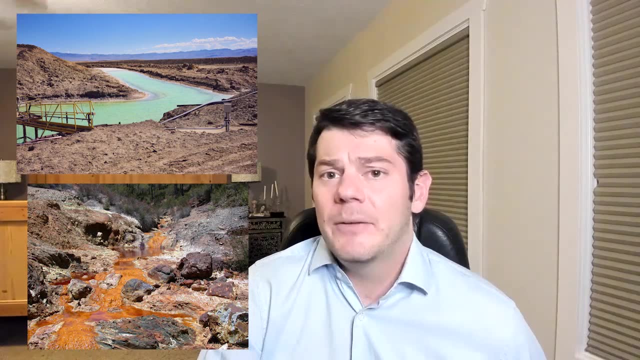 it eventually. The environmental impacts of mining tend to disproportionately fall on certain communities, and that's why I'm here today to talk to you about the environmental impacts of mining. The environmental impacts of mining tend to disproportionately fall on certain communities, such as Native American communities in the United States, so reducing the amount of uranium that we. 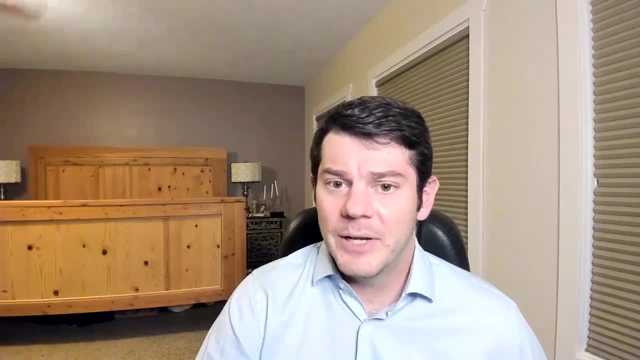 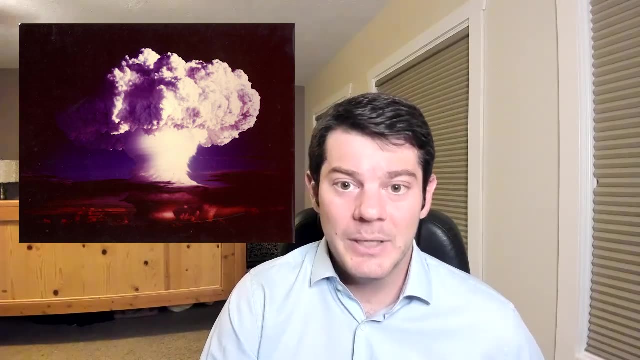 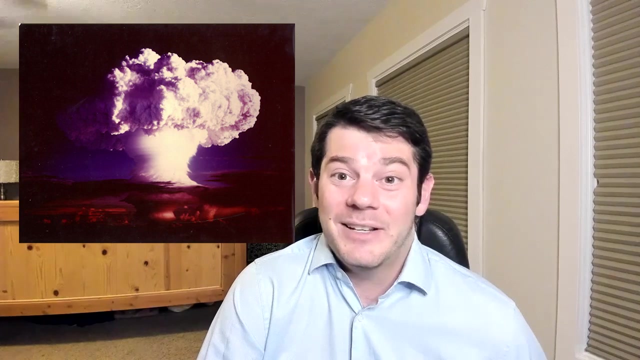 need to mine helps promote energy justice. The other main downside to reprocessing our waste is the possibility of proliferation. When you chemically separate the elements in spent nuclear fuel, you could theoretically divert the plutonium in the fuel and use it to build a nuclear weapon. After all, reprocessing is how we and every other country got the. 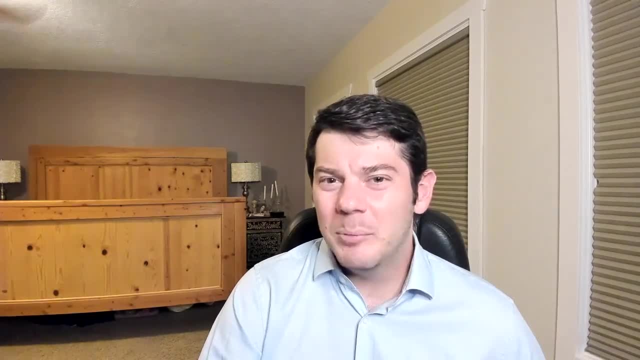 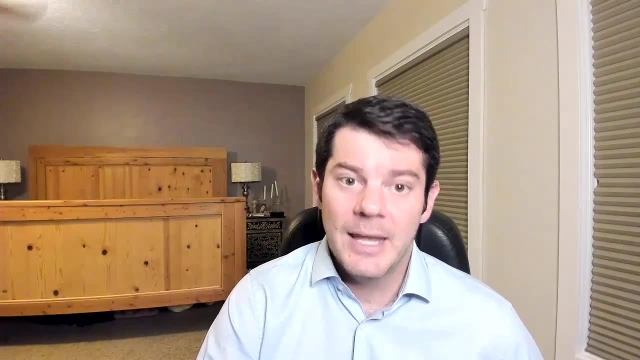 plutonium that we use in nuclear weapons. However, not all plutonium is created equally. Nuclear weapons need to have extremely pure quantities of plutonium-239,, and the plutonium that stays in the reactor tends to sit around too long and tends to accumulate a lot of plutonium-240.. Therefore, reactor-grade plutonium generally performs poorly in nuclear weapons. Understanding why reactor-grade plutonium is bad for nuclear weapons crosses the red line into nuclear weapon design, which of course is classified material. But what the heck? 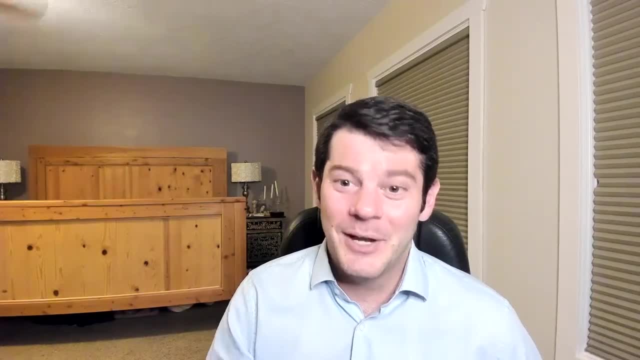 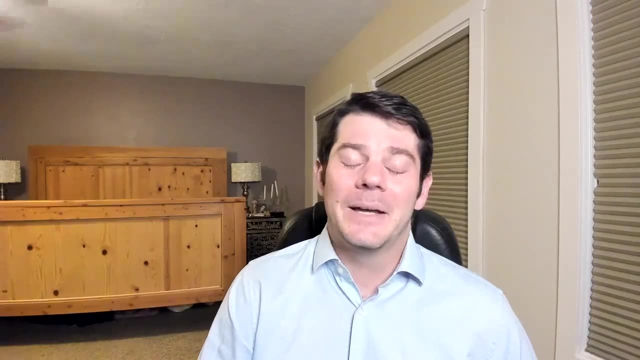 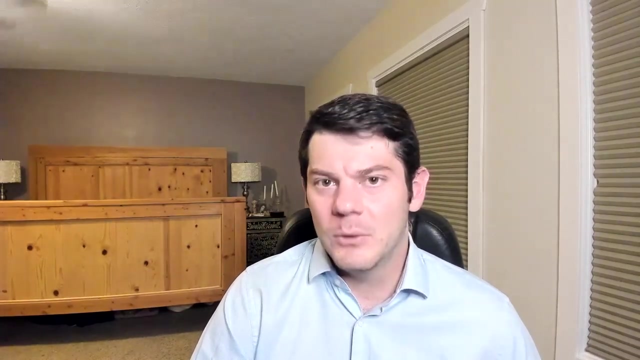 I need to get this channel monetized. I need to get more likes and more subscribes. so let's discuss nuclear weapon design, You see. Anyway, the general sense in the nuclear engineering community is that reactor-grade plutonium is not super effective in nuclear weapons. So reprocessing our spent nuclear fuel, 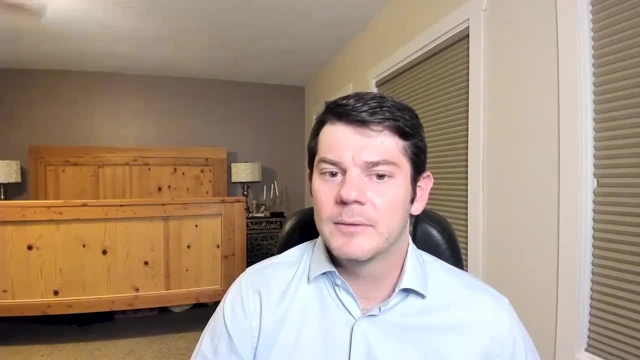 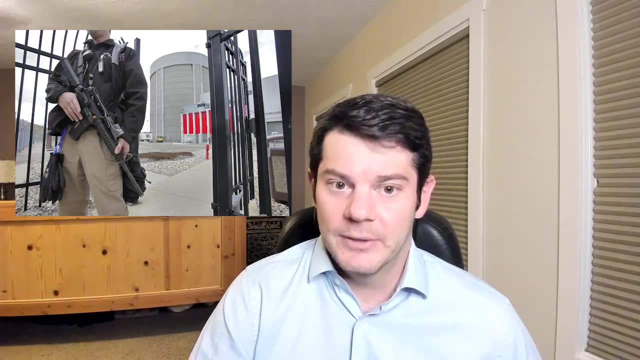 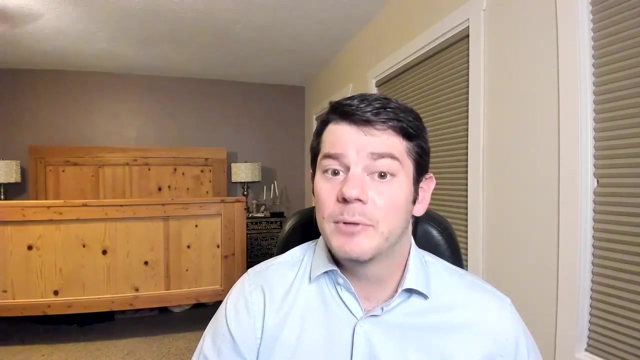 doesn't create as many proliferation concerns as you might think. What's more, reprocessing is likely to take place in a centralized location with a lot of guards and a lot of guns, So breaking into a reprocessing facility won't be easy. And even if you could break in, the actual reprocessing 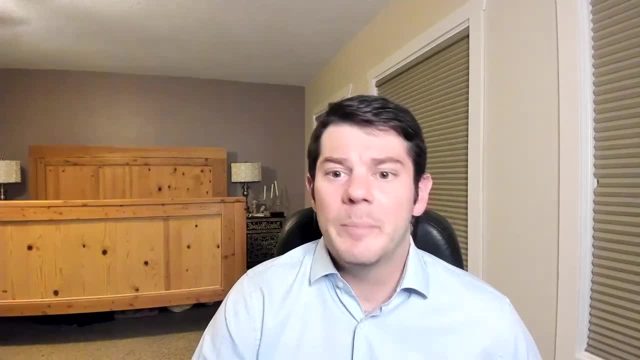 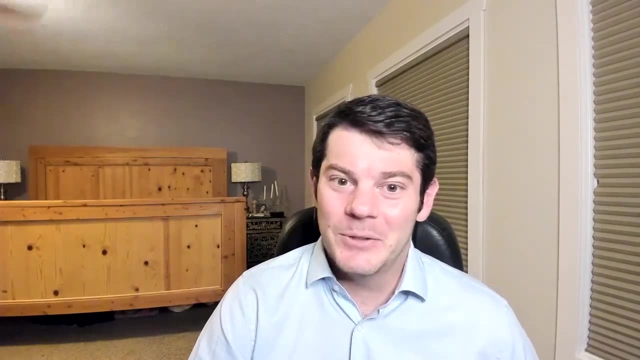 process is likely to either take place remotely or behind glove boxes because of the enormous dose that you would get from standing next to spent nuclear fuel. So good luck figuring out how to break into a reprocessing facility and figuring out how to pilfer the plutonium without instantly. 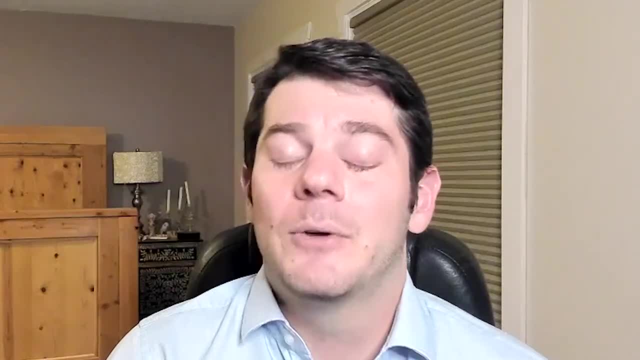 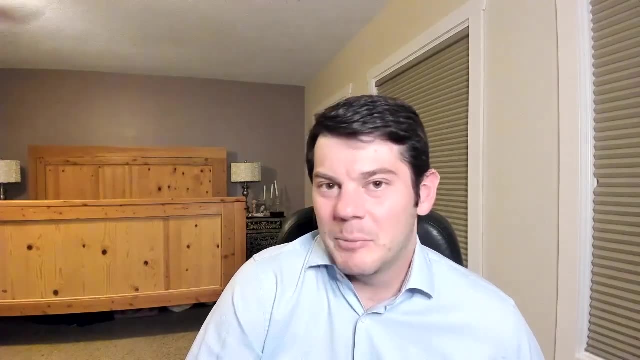 getting a super-fatal dose of radiation or a super-fatal dose of bullets And remember all this time and effort to steal the plutonium might make a very small, maybe usable nuclear bomb If you're a terrorist who just wants to. destroy things. C4 and conventional explosives already do a great job of blowing things up, And if you really just want to make a nuclear weapon, a gun-type nuclear weapon using enriched uranium works just fine. You can extract uranium from seawater and it might be easier to get. uranium, enrich it and make a uranium nuclear weapon than it is to plan a suicidal heist to get plutonium from a reprocessing plant. So, personally, stealing plutonium sounds like a lot of work for not a lot of gain. Nonetheless, reprocessing spooks quite a few people just because of the possibility of nuclear. 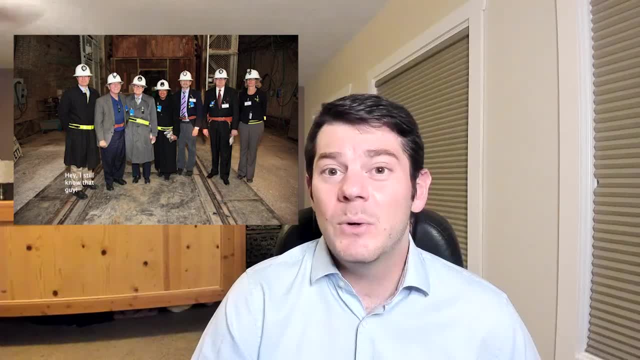 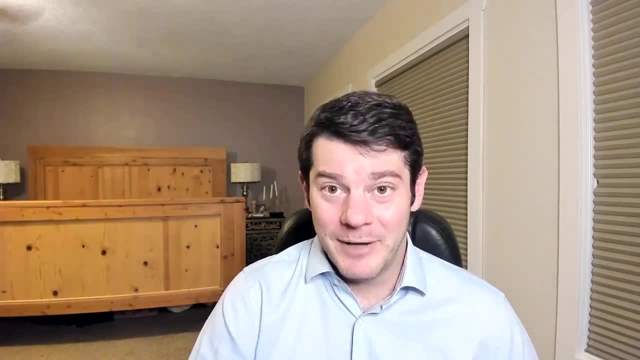 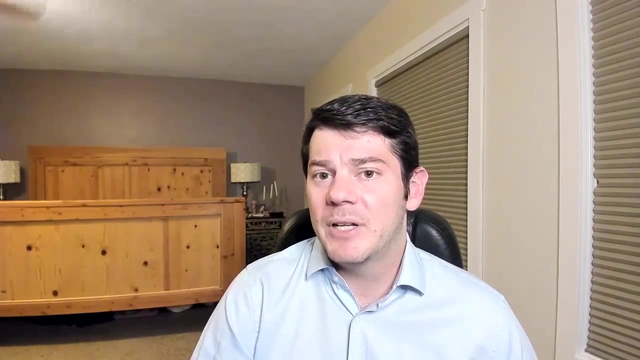 proliferation, to the point that the Blue Ribbon Commission was actually split on whether or not we should reprocess our spent nuclear fuel. Anyway, this concludes our video on reprocessing. Reprocessing is probably my personal favorite option for disposing of nuclear waste, both because of how much it can reduce the volume of spent nuclear fuel. and also because of all the other benefits you can get out of the spent nuclear fuel. The risks of reprocessing are, in my opinion, small and can be mitigated, and putting unreprocessed spent fuel in a geological repository just throws away so many valuable medical isotopes. Right now, reprocessing is not the most economic option.